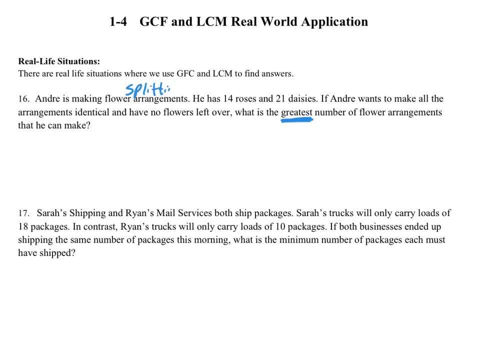 into groups. So we're splitting into groups, And that's what factoring does. Factoring pulls a number apart into groups that when we multiply them together we get back the original number. We can kind of think about it that way. So those are two things that 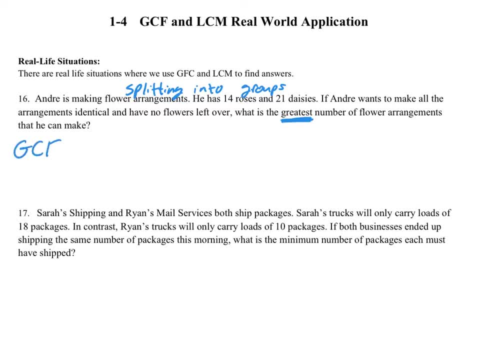 we can think of. that will clue us in to this being a greatest common factor problem. So we have 14 roses and 21 daisies. We're going to start by finding the GCF of those guys So we can start with a prime factorization. 14 is really two times seven And 21 is really. 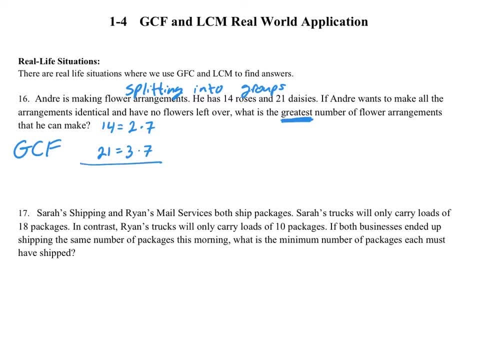 three times seven. So when we find a GCF, we only take the common factors. So they both have a seven in common. So that's what we're going to pull down. Okay, So what this seven tells me is: I can make seven arrangements. All right, And what would these arrangements? 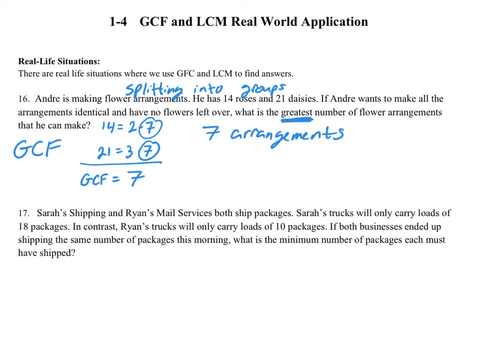 look like Okay. So if I made seven arrangements and I have 14 roses, that means I'm taking those 14 roses and splitting them up into seven flower arrangements, So each arrangement would have two roses. And then we're taking 21 daisies and we're splitting those up evenly. between seven arrangements, So 21 daisies. And then we're splitting those up evenly between seven arrangements, So 21 daisies. And then we're splitting those up evenly between seven arrangements, So 21 daisies. And then we're splitting those up evenly. 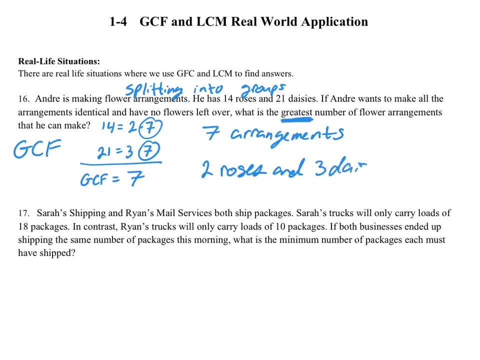 by seven is three, So we'd have three daisies. All right, So Andre could make seven arrangements, And those arrangements would have two roses and three daisies. It only really asks you about the number of arrangements, though, So the two roses and three daisies. 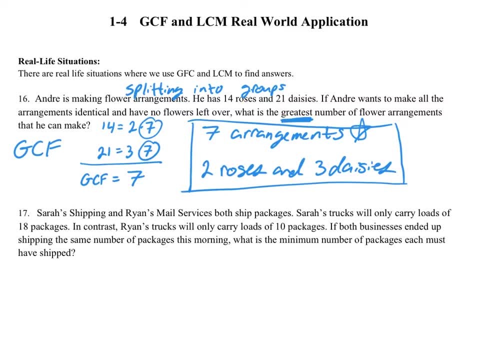 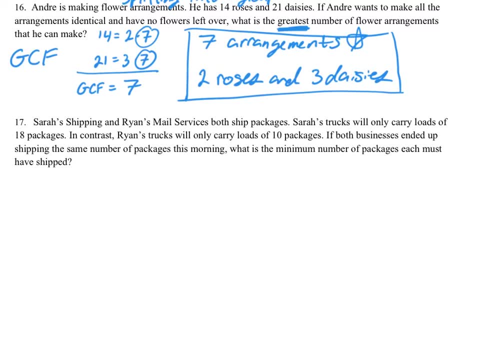 information is just bonus for us, Okay. 17. Sara's shipping and Ryan's mail service: both are vogelack packages. Sara's truck will only carry loads of roses And her mail service of 18 packages. In contrast, Ryan's truck will only carry loads of 10 packages If both businesses 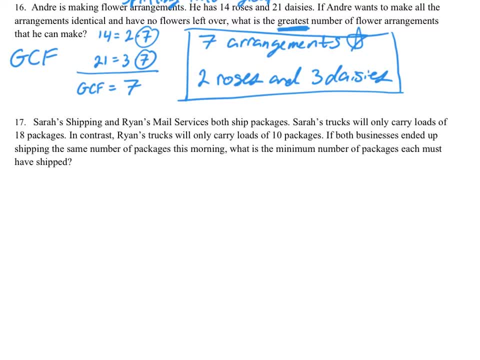 end up shipping the same number of packages this morning. what is the minimum number of packages each must have shipped? Okay, so let's talk about whether this is GCF or LCM. So again, kind of a cue word that we can use is minimum, right? So GCF is the greatest, LCM is the least. 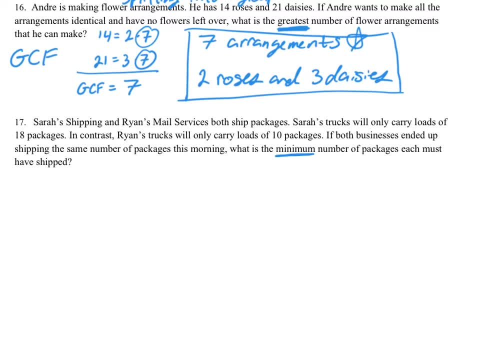 So when we're talking about minimum or smallest, we want to be looking at LCM. Another thing that we might want to think about is how many packages we will be shipping, right. So, Sarah, will she ever ship less than 18 packages? She will not. It says she carries. 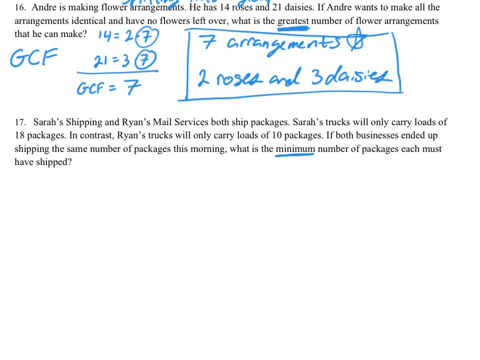 loads of 18 packages, which means she's either going to be at 18, or, if she does two shipments, she'll be larger than 18.. So least common multiples are always 18.. So if she does two shipments, she'll be larger than 18.. So least common multiples are always: 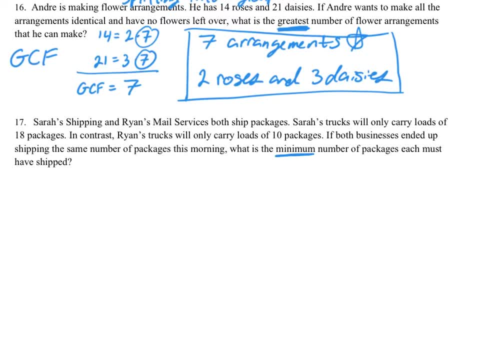 18.. So if she does two shipments she'll be larger than 18.. So least common multiples are always greater than or equal to okay, So we want to think about that. So this is going to be an LCM problem. So that means we need to find the least common multiple of these packages being shipped. 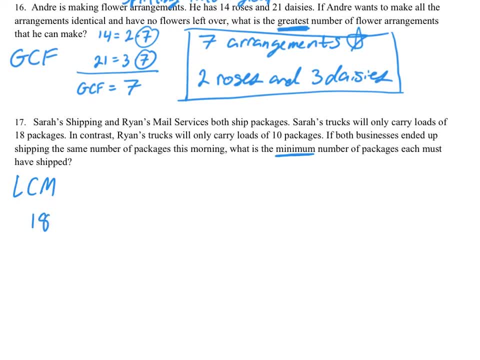 So where Sarah is starting with one shipment of 18 packages and Ryan starts with one shipment of 10 packages, all right, So then Sarah does a second shipment and now she's shipped 36.. Ryan does a second shipment and now he's shipped 20.. So we're going to keep up this pattern and we're going to see at what. 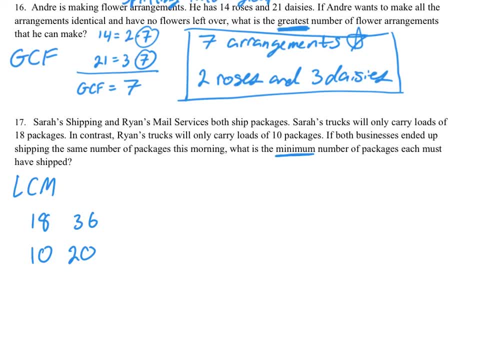 point, do they meet up? So if Sarah does another, then she's at 54.. Ryan would be at 30.. All right, and we want to keep going. So if Sarah does another, she would be at 72.. Ryan would be at 40.. 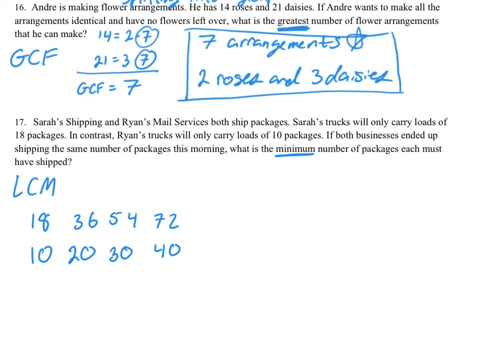 And another. we would have Sarah at 90, and Ryan at 50. Now you might notice something about 90. You might notice that 90 is divisible by 10, and you might want to stop there and that's fine.